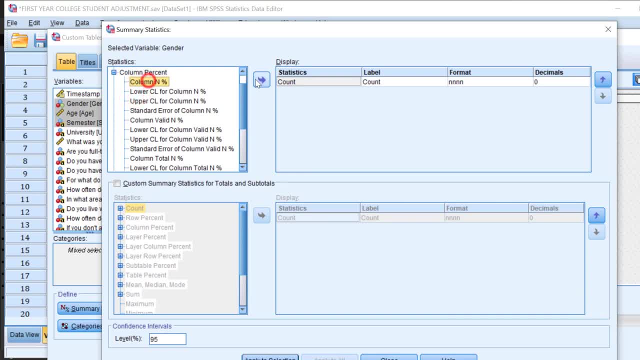 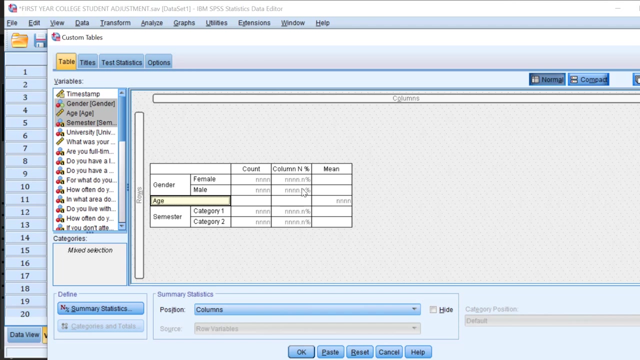 for instance uh, column percent, and move it here, then click apply to selection- the same method can be reapplied here And then close. so once I do this, so for age, I may add: since it's uh, so for age, since it is, let's say, a continuous variable, we need a mean score and standard deviation, let's say value. 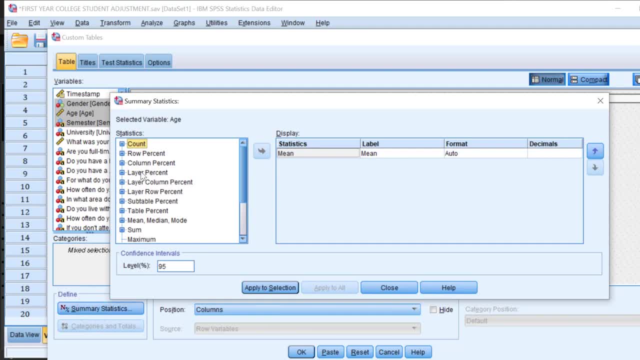 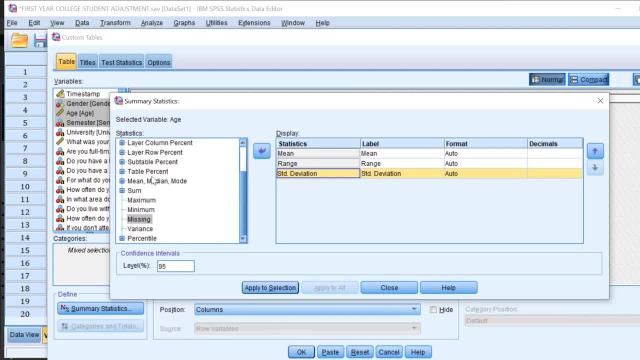 So I'm going to go again to summary stats and I'm going to move, for instance, the range and the standard deviation. I can even have the variance and the percentile if I want the mean median and mode. let's just do this as well. so let's remove this so that I can. 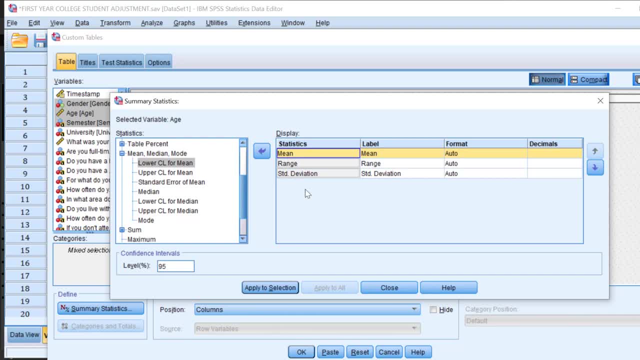 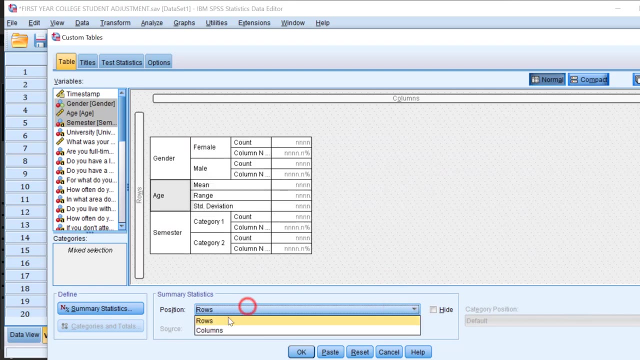 okay. so let's go back to this mean and put it first. so, as I said, I can include also the mean median and mode. so so I can include one by one, apply to selection, close, and then I can just change here how the table looks like. so we'll keep it this way and click. 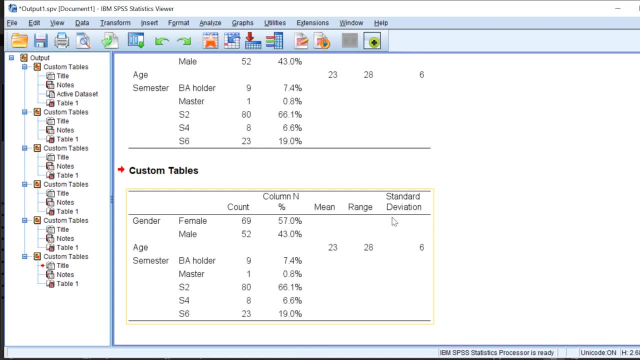 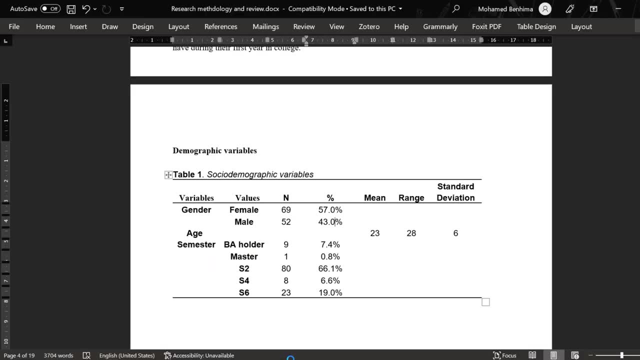 okay and wait for the output. so here is the output. so what I can know, uh can do now is that copy this output and paste it to Microsoft office word and format it this way. so this is, in brief, how we can combine demographic or social demographic variables into one personalized 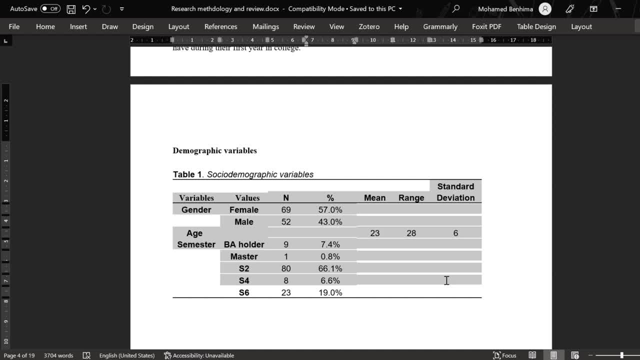 table without having to do a lot of manual work, and we can do this effectively using SPSS. if you have questions or remarks, do not hesitate to post them below or contact me honestly. I answer as many inquiries as possible, depending on my availability. if you can contact me via whatsapp, it's more convenient for me to respond on the spot. 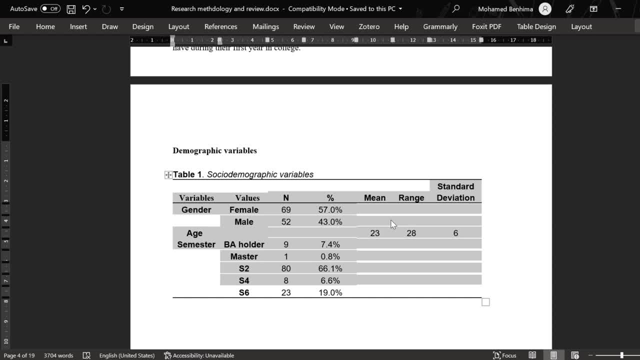 otherwise, if you use email or you can comment here below the video. it's also good because I keep checking every now and then, so I always have my internet connection on and I can react as as soon as possible. uh, thank you so much. I really do learn from.